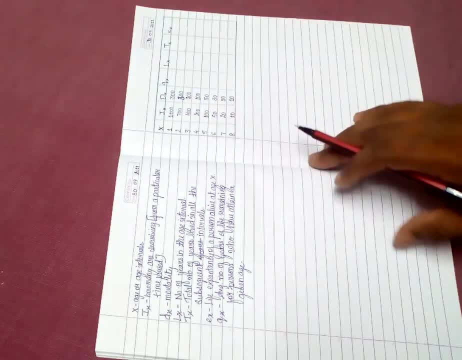 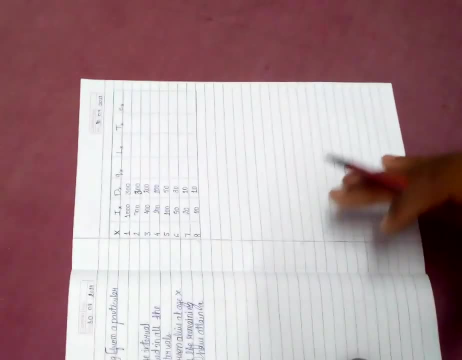 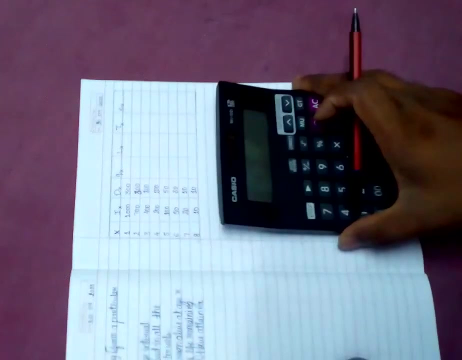 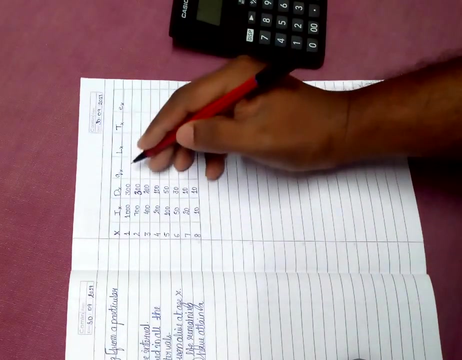 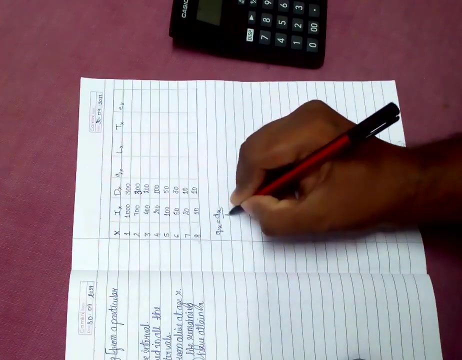 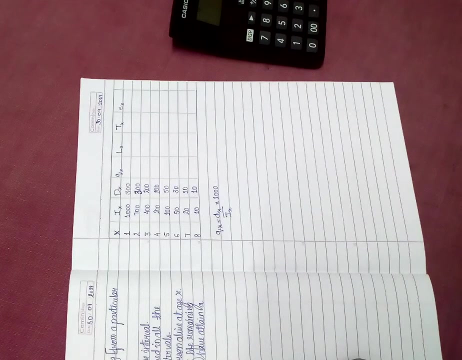 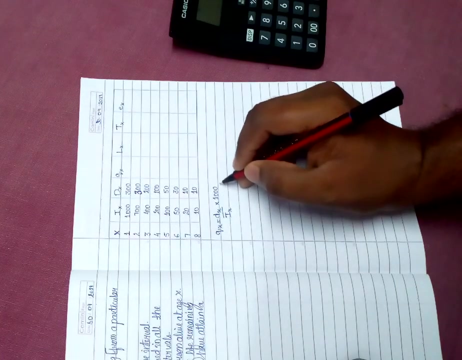 the mortality. so over here, as you can see, wait a second. yeah. so over here, as you can see, for this experiment to be conducted we require calculator. so first of all, Q X. we are going to calculate Q X by. Q X is equal to DX upon IX into thousand. okay, so Q X is calculated DX upon IX multiplied by. 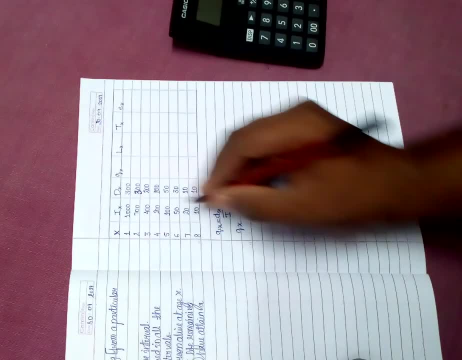 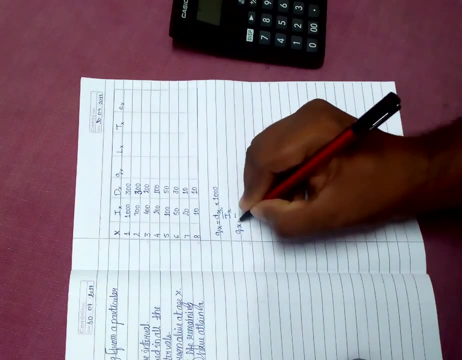 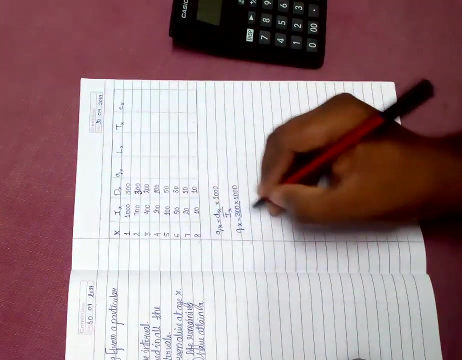 thousand. so first of all Q X for the first value. let us take the DX value. DX, it is equal to 300 into 1000. it is equal to 300 into 1000. so this is the value divided by the IX value, that is 1000. 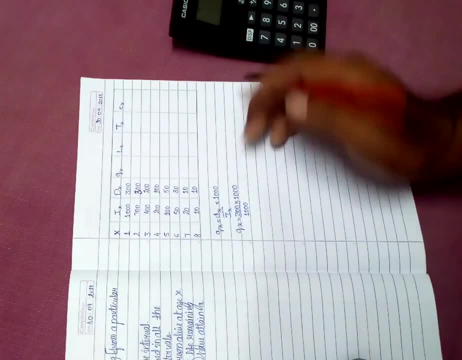 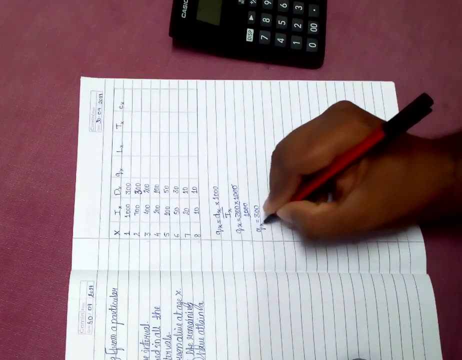 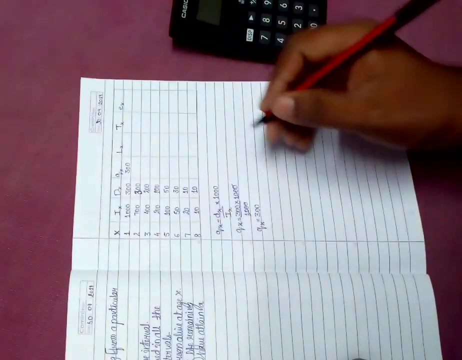 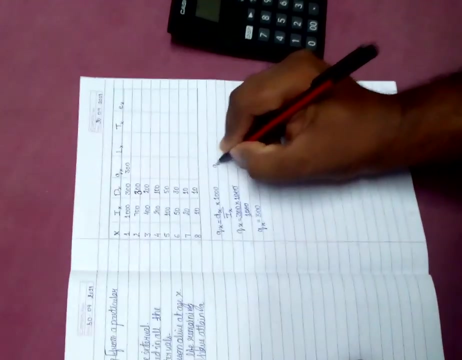 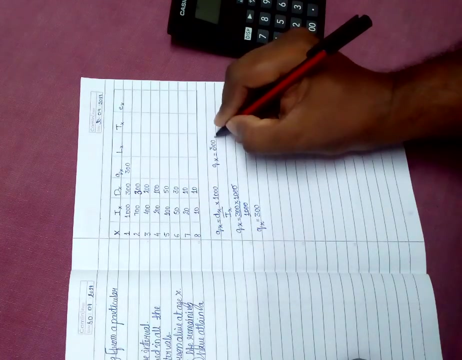 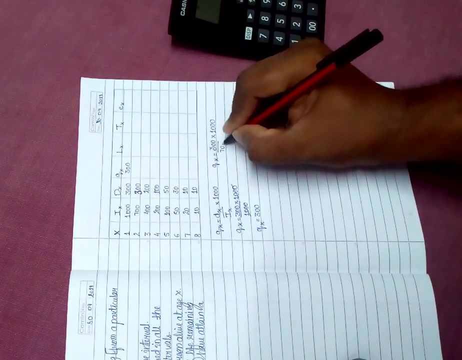 so Dev Przy dot. so this is simple calculation for this video. require push manufacture shelves and this it comes to 300 for the first of Q X. so Q X for the second one will be 300 x 1000 divided by 700. so if we 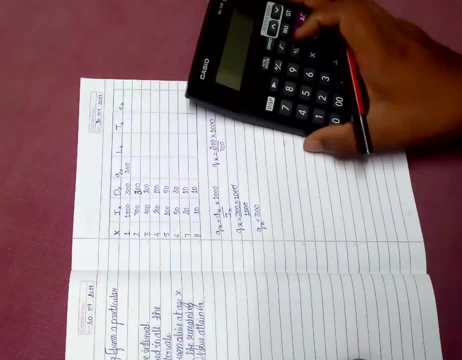 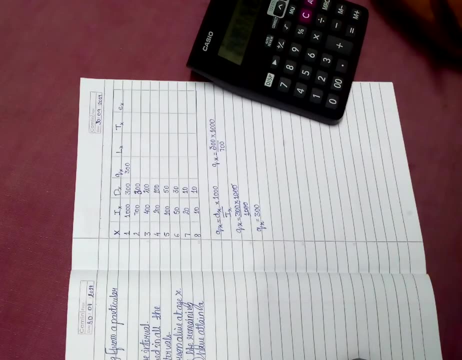 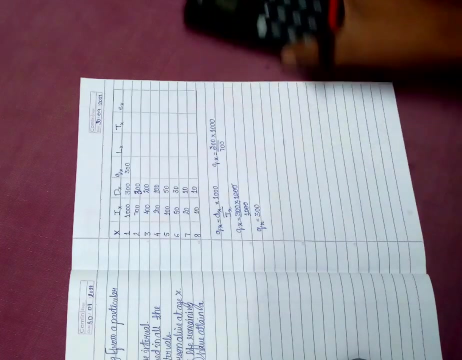 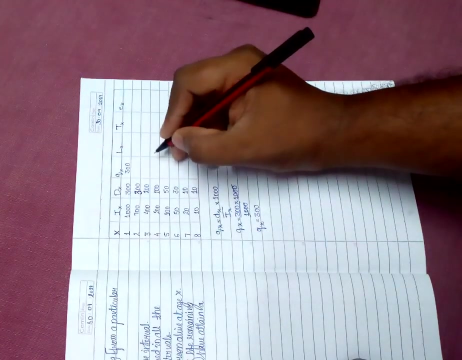 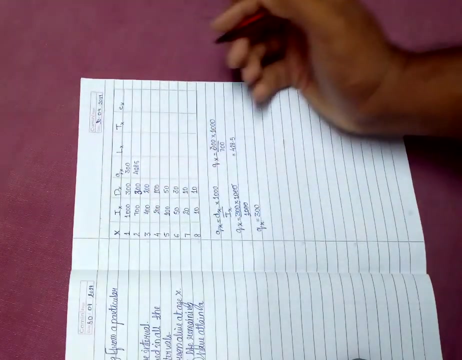 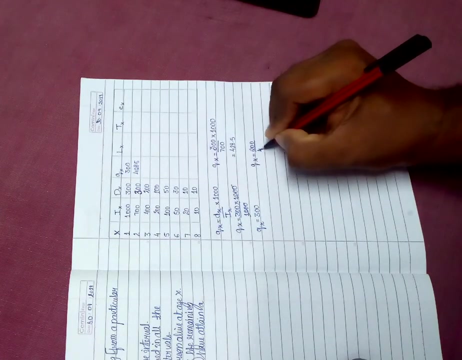 calculate this by using calculator. that is: 300 divided by 700 into thousand, it comes to four twenty eight point five. it comes to four twenty eight point five, so we are going to write it for twenty eight point five. then by doing this for the third one, Q, X is equal to 200 by 400 into thousand. so it 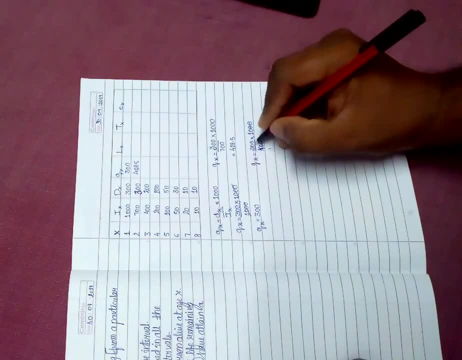 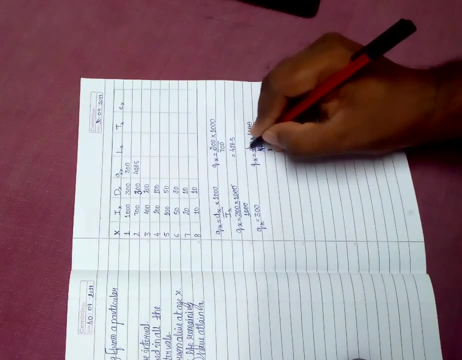 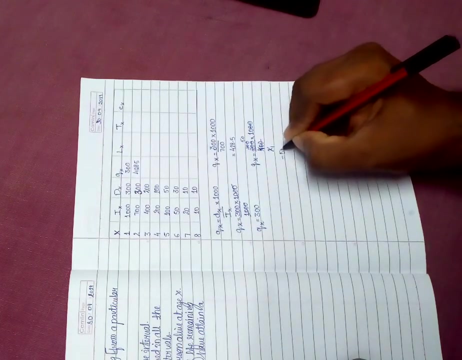 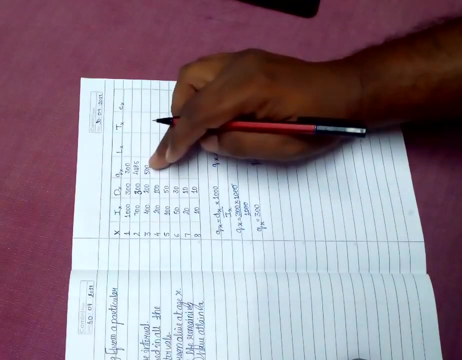 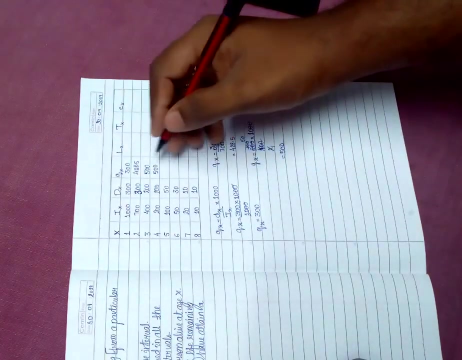 will come approx around for one the two, so it is coming around to five hundred. so over here it is five hundred. okay, so now we are going to calculate for this, so it will come to five hundred. I'm not doing the calculation because this will take a long time for me to this video, so hope. 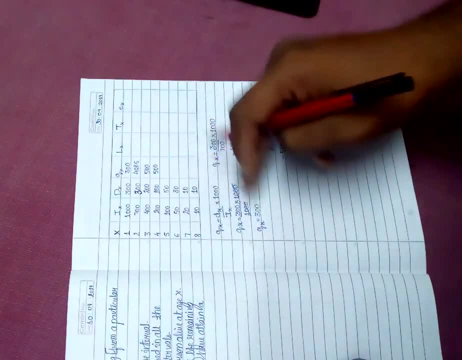 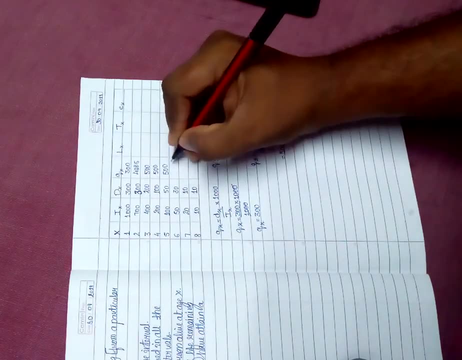 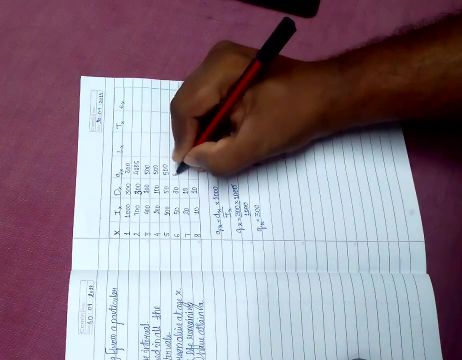 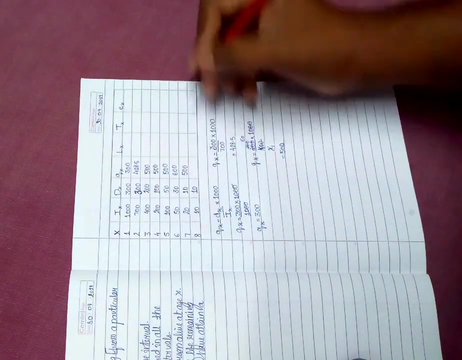 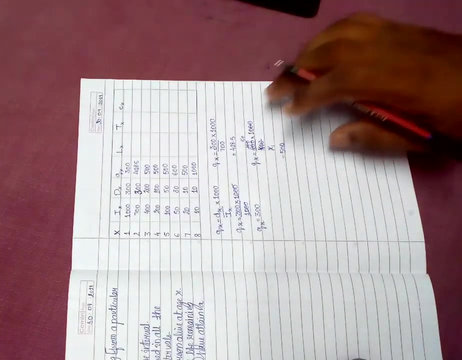 you'll have understood this calculation. if you have not understood, please replay the video. okay, so this will be also picture of this. so we are going to go to End, End. so this will be 600, and this will be five hundred, and then 1010, so this will be 1000. so okay, so now we are done with theisms. 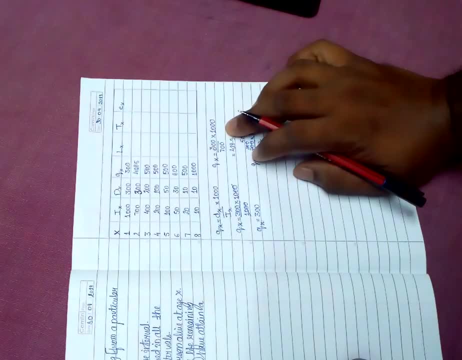 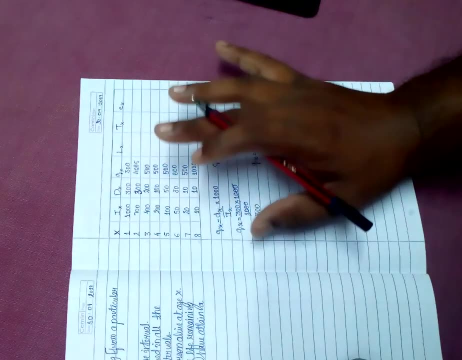 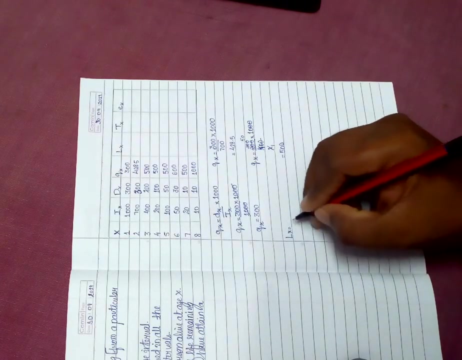 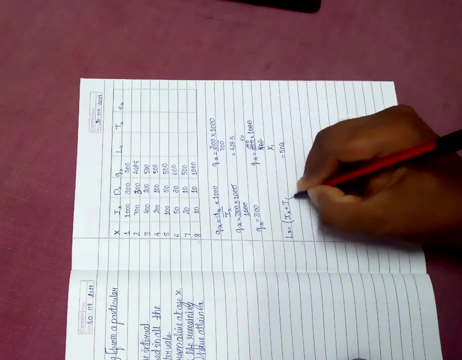 We beat the Skidoding in dis candidates with the Здесь. we beat the Skidoding in dis candidates Q, X value. so hope you have understood this QX part. so now we are going to do LX column. so the basic formula for LX is equal to IX plus IX plus 1, the entire thing divided. 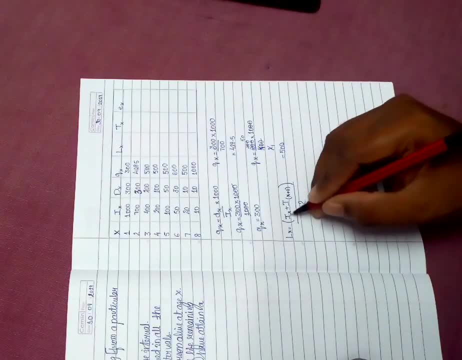 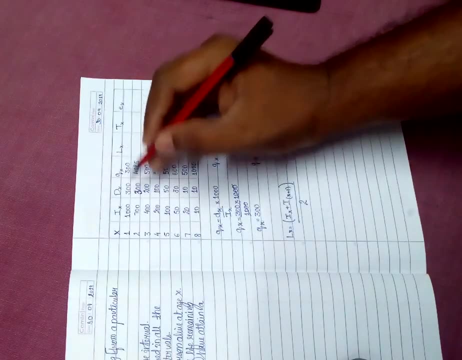 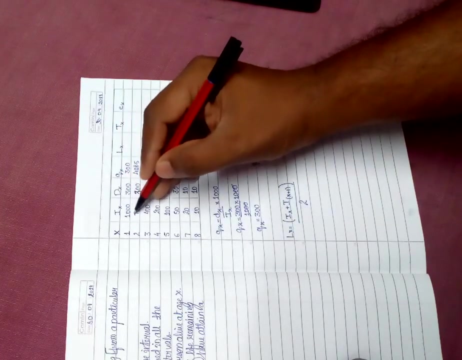 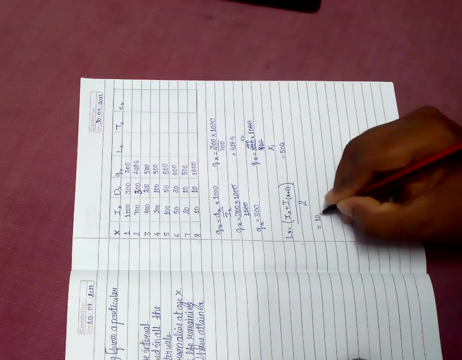 by 2. okay, special what I X suppose say for this column. if we are doing the LX value, okay, so IX over here will be this value and I explain: swan will be this value. okay, what it. so for here it will be first one: I am doing 1,000 plus 700. 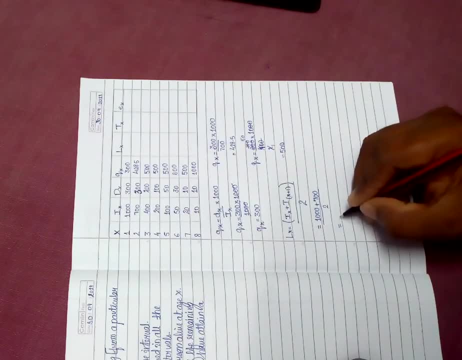 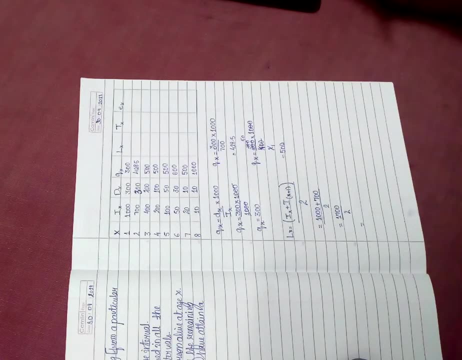 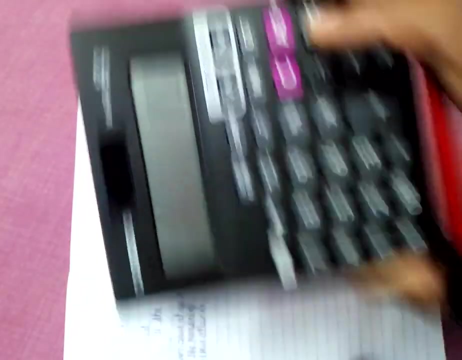 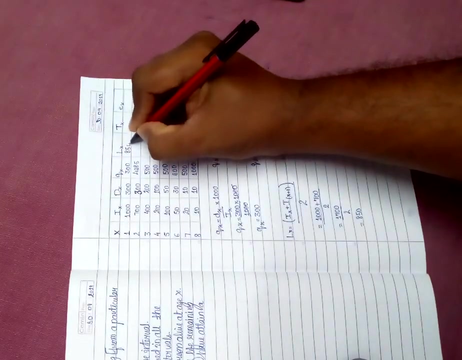 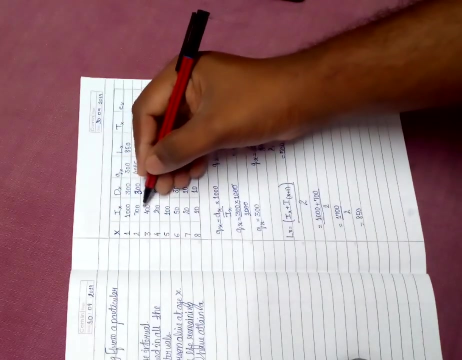 pond 2 comes to 1700 divided by 2. if you calculate it 1700 divided by 2, you get 850. okay, 850. so the first value over here will be 850. then if you add subsequently the other numbers, 700, 700 plus 400 and just show your calculator, 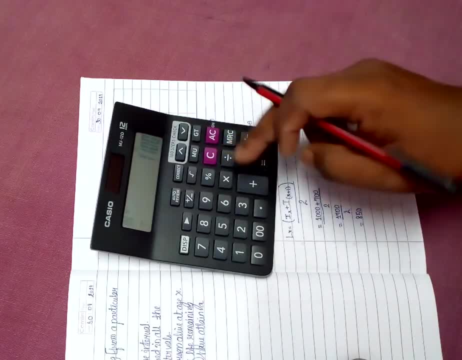 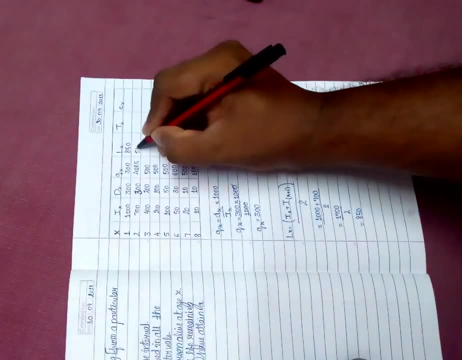 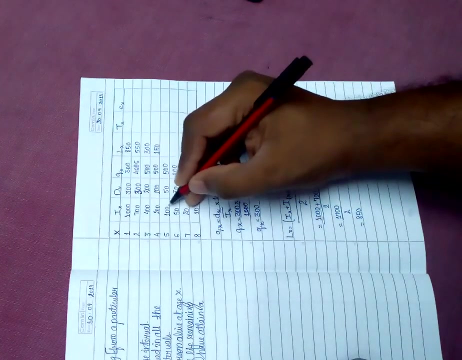 700 plus 400 equals 2 divided by 2 comes to 550. okay, so this will be 550, okay. then 600 divided by 2, that comes to 300. divided by 2, it comes to 150, then 150. divided by 2, it comes to 75, then 35. 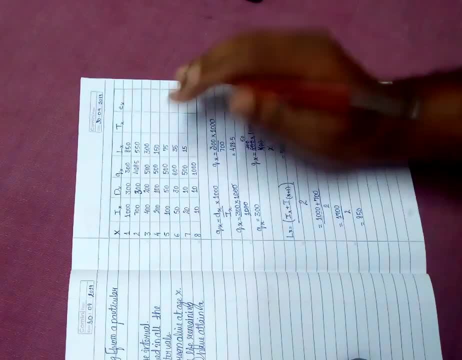 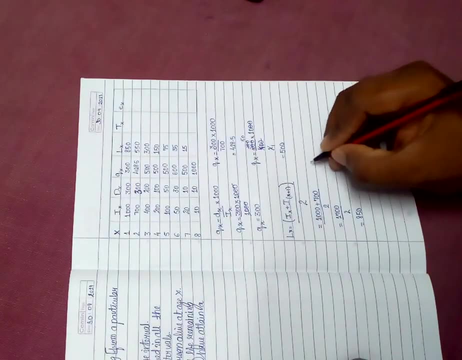 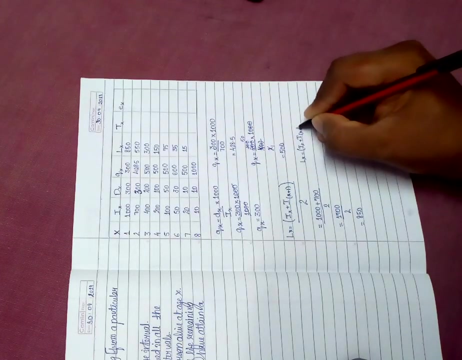 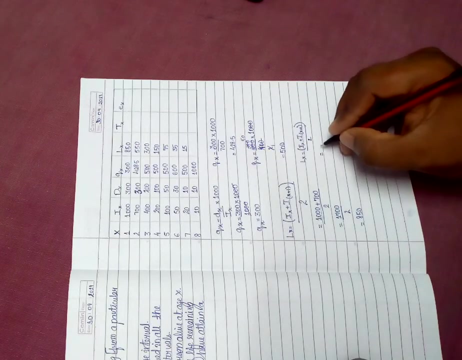 then 15. okay, so now over here you will get consumed confused, okay, so over here what we do is: over here, we take: LX is equal to I X plus I X plus 1 divided by 2. okay, so over here what we do is: I X value is: 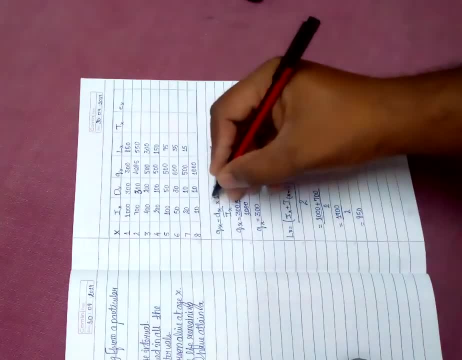 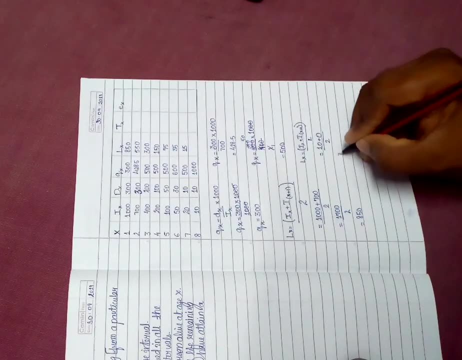 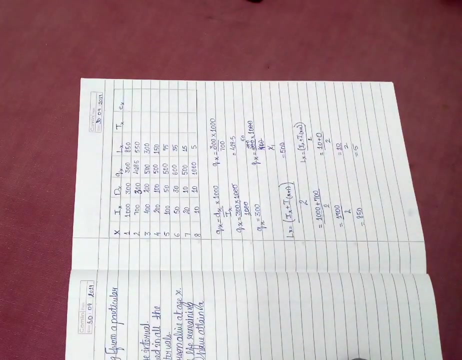 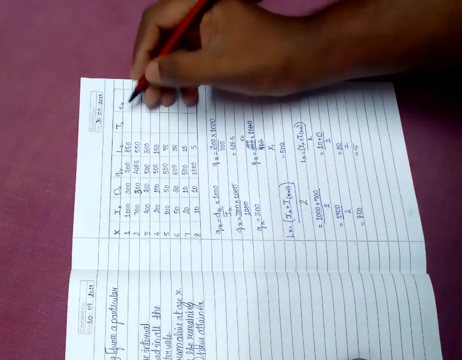 taken as 10 plus 0. see, because after this there is no more row, okay, there are two. it comes to 10 divided by 2, that will be equal to 5, okay, so this will be 5, so now. so now we are going to do the DX. 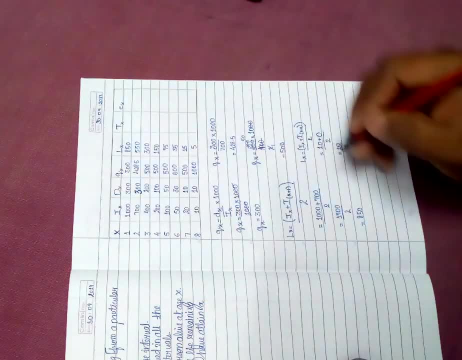 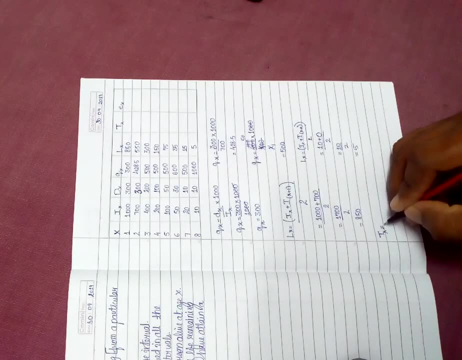 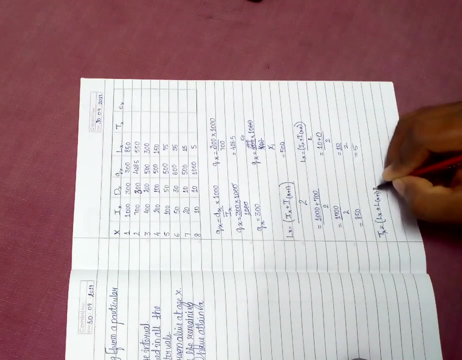 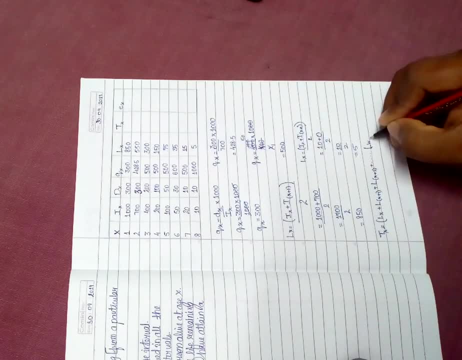 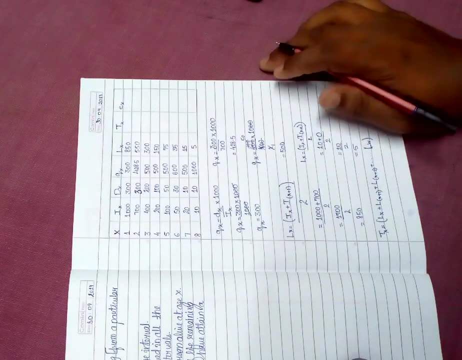 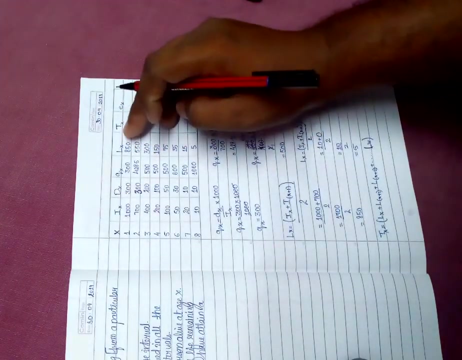 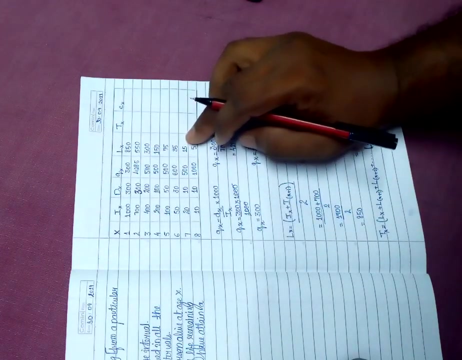 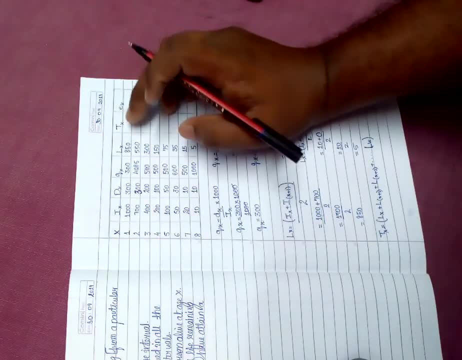 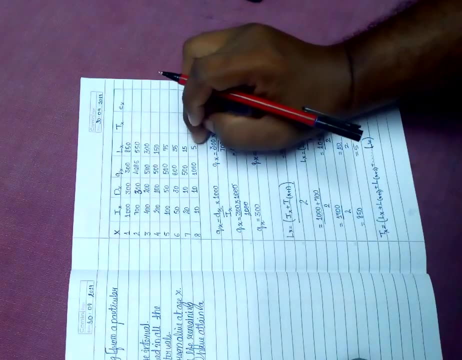 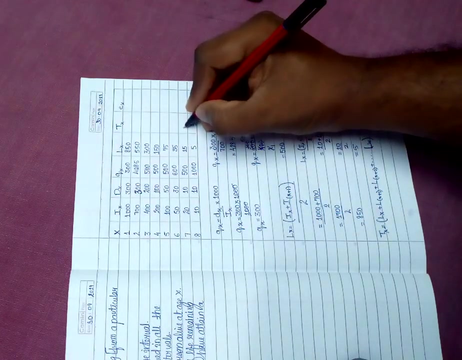 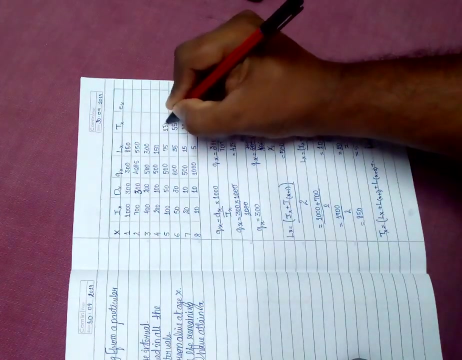 all. minus this, then find this- this is another way- then minus both of this and find this okay. so, and another way is go this way. so I'm going to go this way. so it will be 5. 5 plus 15 is how much? 20, 20 plus 35, it is 55, then 130, then 280, then 5. 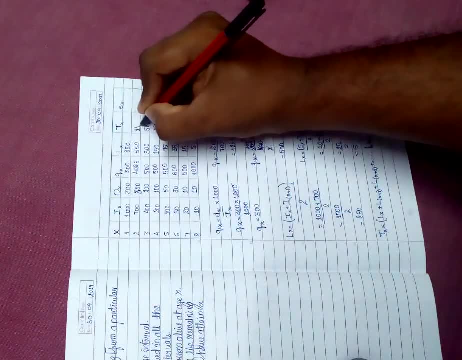 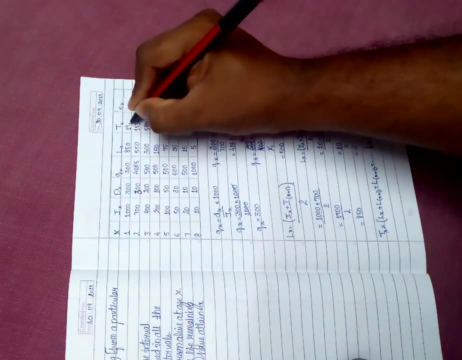 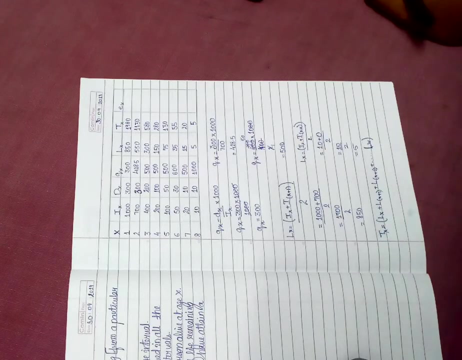 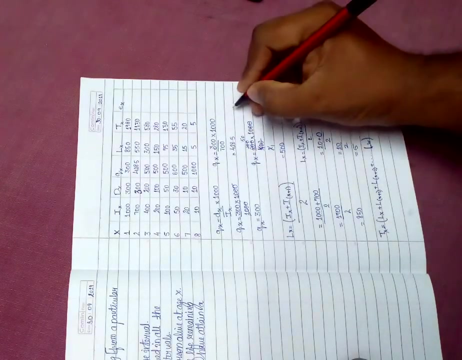 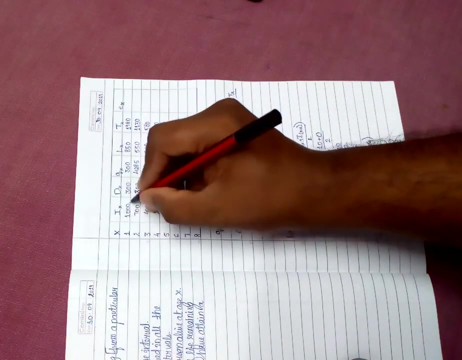 80, then 1130, then it will be okay. one nine, eight, zero, okay. so this tx column is done, finally. so finally, the main thing is up. it's the e X, X is what we require to calculate. so the main formula, formula that is used for Ex is Ex is equal to Tx, this Tx upon the Ix. so I will explain. 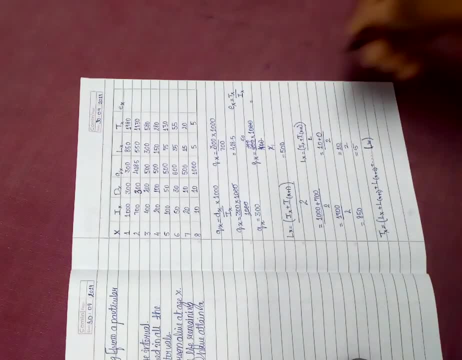 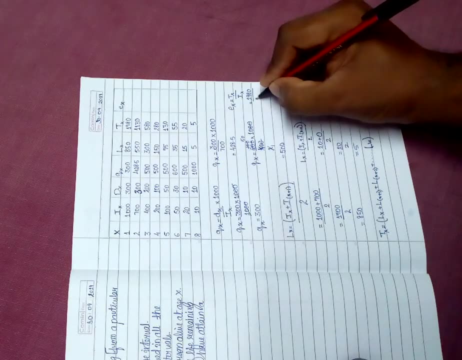 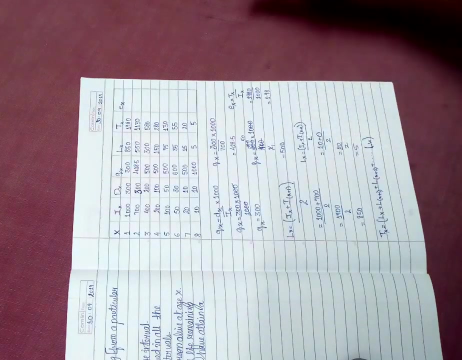 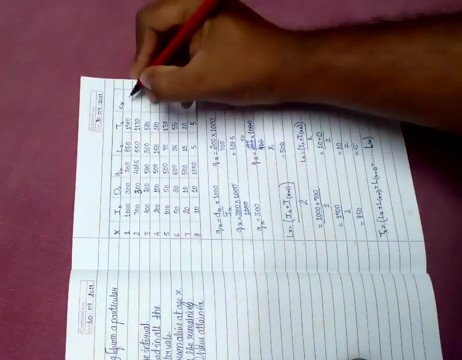 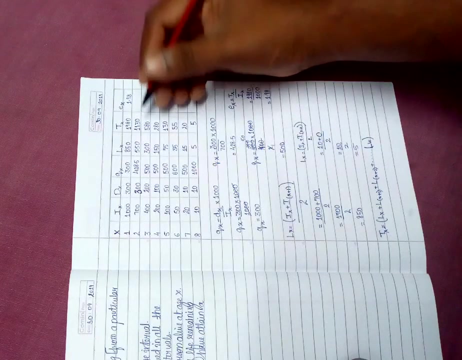 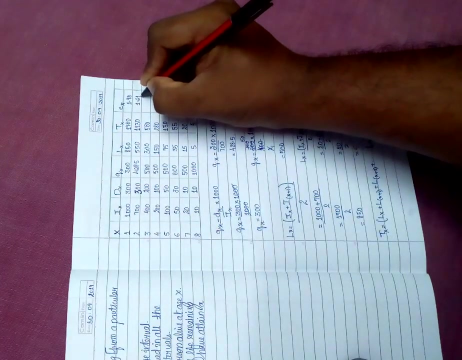 over here the first one. so the first one. values are 1980 divided by 1000, so it will be one point nine. you can calculate over here with the help of calculator, so this will be one point nine eight. so then if you divide by this the second one, 1130 divided by 700, it comes to 1.61, then 1.45. I'm not going to calculate this. 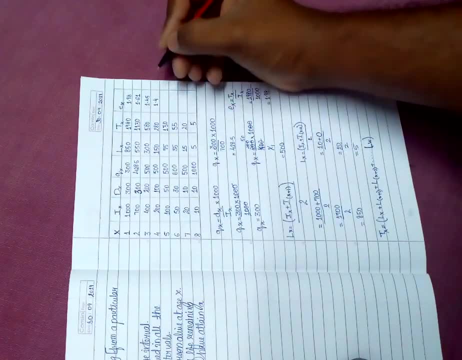 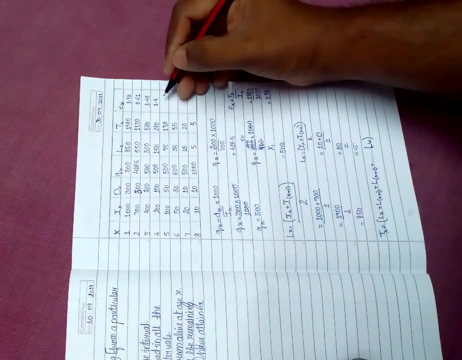 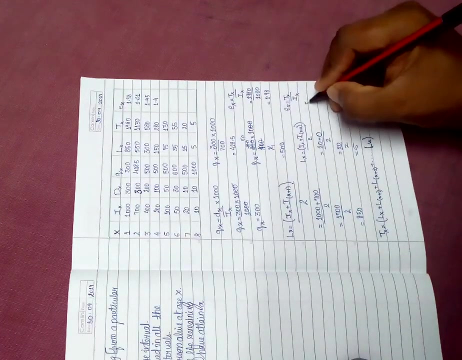 if you all want to see, you can see this calculation. if you have not understood, you can replay it or I'll do it for another one now. Ex is equal to Tx upon Ix. okay, listen carefully here. Tx, it is 130 divided by 100. okay, so let me use this: 130 divided by 100. 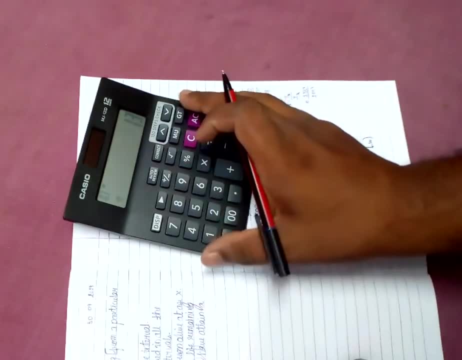 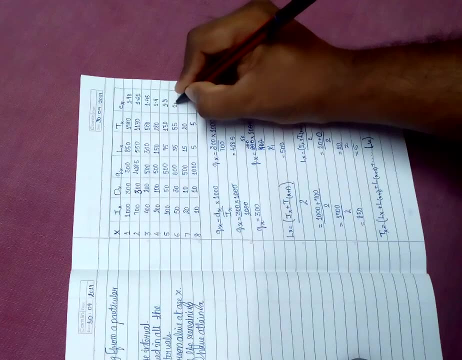 130 divided by 100, it comes to 1.3. okay, hope you have got it. 1.3 then 1.155 divided by 5. so if I calculate this again, Tx, I am going to calculate this by 100. so 1.35 divided by 100. 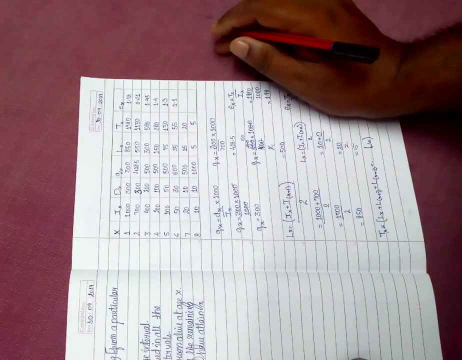 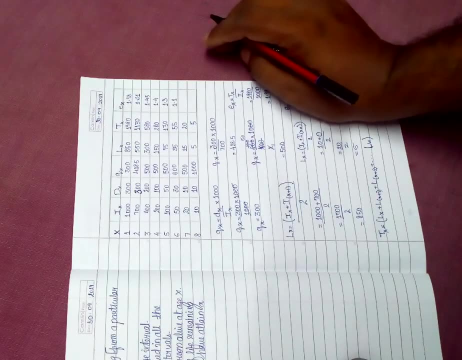 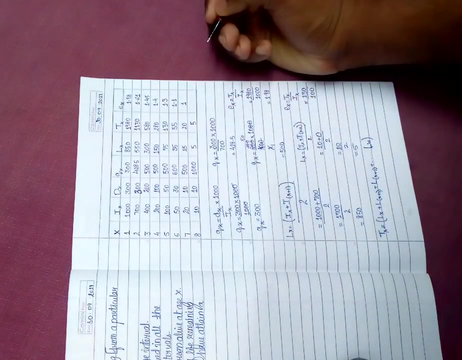 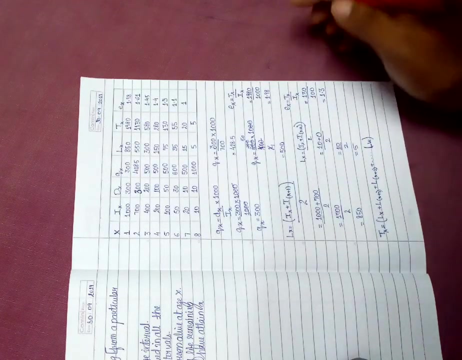 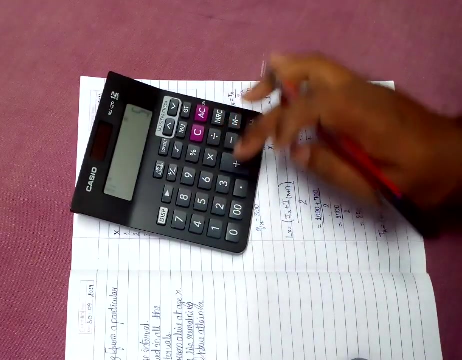 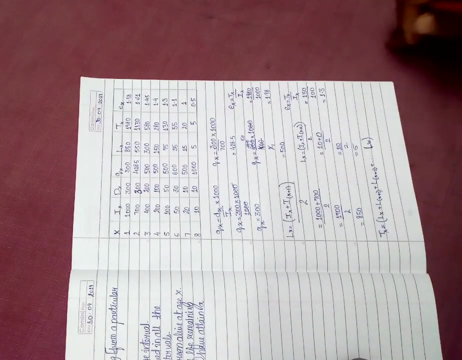 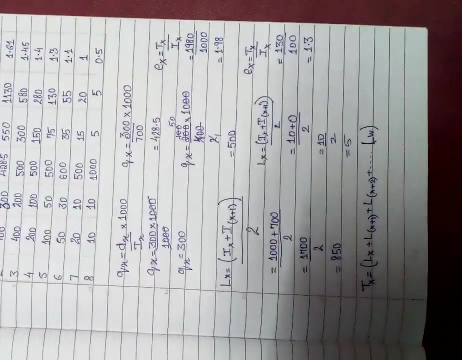 see over here: 20 divided by 20: okay. 20 divided by 20, how much one? okay, 20 divided by 20: 1. right then. 5 divided by 10 is equal to 5 divided by 10 is equal to 0.5. okay, so let me zoom the video. I mean, if you want, you can take a. 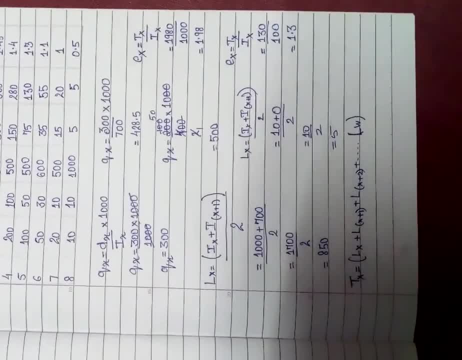 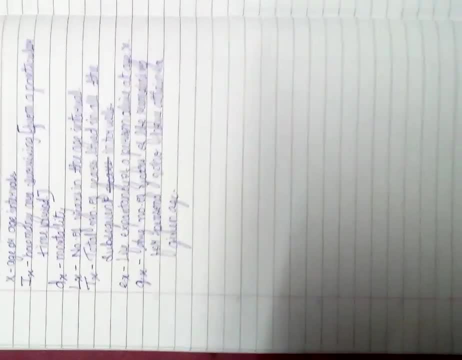 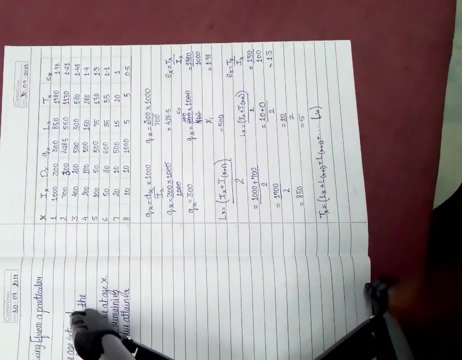 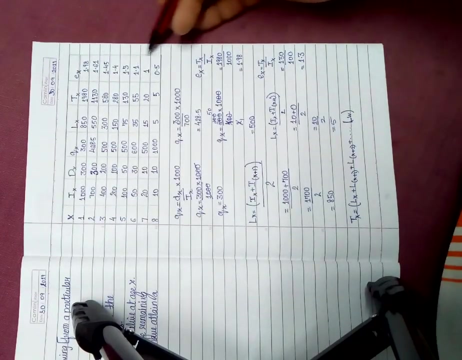 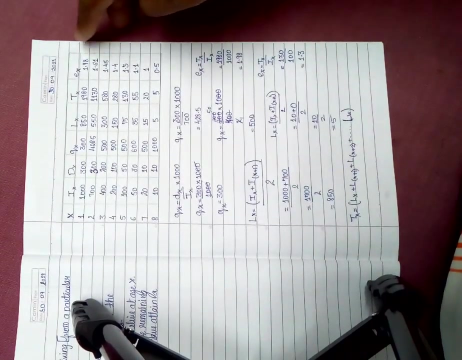 screenshot and try to understand this. so this was this also. so this was the hypothetical life table that we are taken to find the life expectancy. so over here, as you can see, the life expectancy goes on decreasing, that is, as the age of an individual, of a specific species. 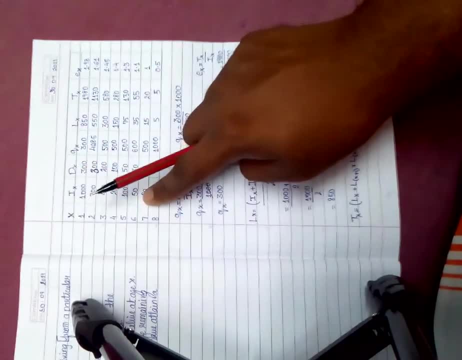 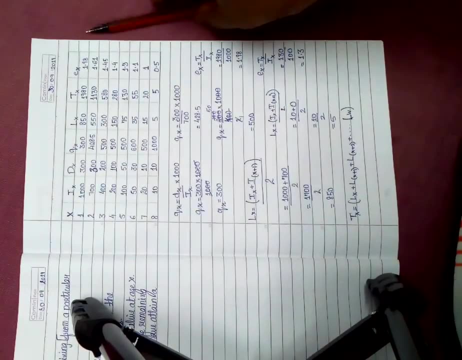 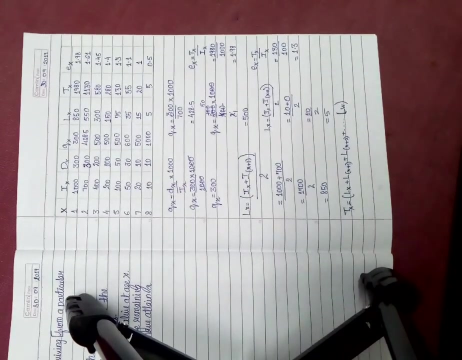 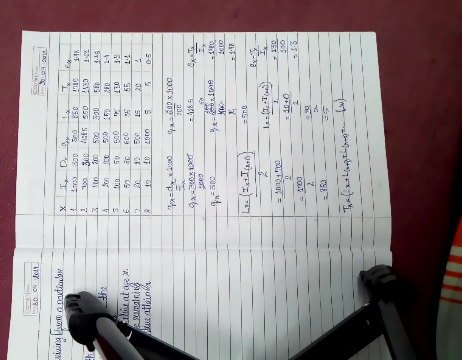 increases age increases the life expectancy of an individual that particular species goes on decreasing. so hope you all have understood the video. so thank you for watching this video. have a nice day. and if you all have not understood anything, please comment below in the comment section and like.